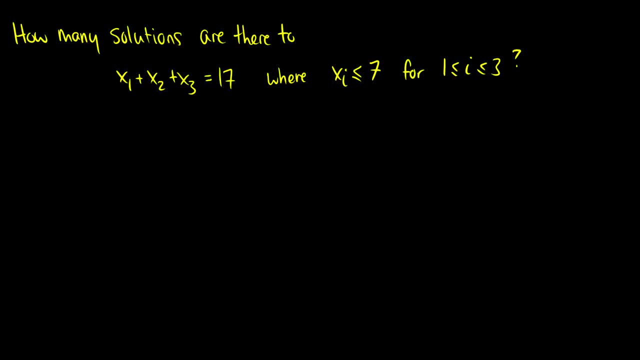 then attempt the last one on your own to make sure you get what's going on. So first question: how many solutions are there to? x1 plus x2 plus x3 is equal to 17, where all of our xi's have to be less than or equal to 7? So this is different Before, when we have, say, 2 has to be less than. 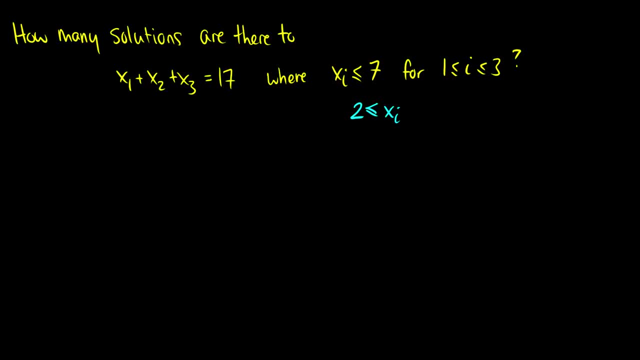 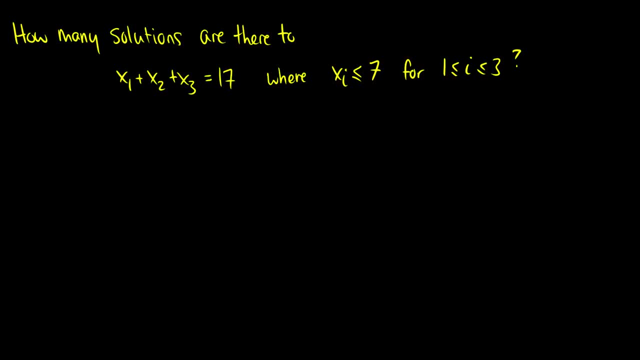 need to do something a little bit different. So what we want really is we want to have the negation of three different conditions to solve this problem. So what we're going to do for our conditions is we're going to say, for all of our conditions, here we're going to have xi. 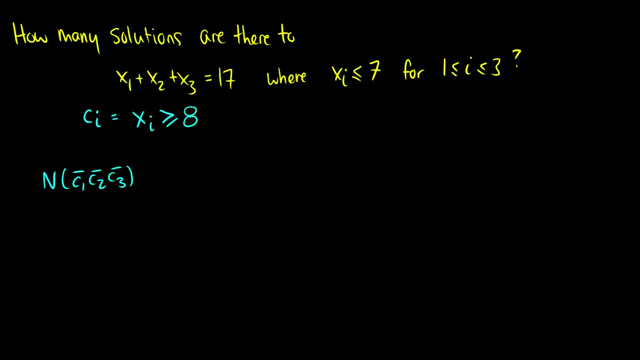 is greater than or equal to 8, because if this is not the case, then not ci is going to be xi less than 8, which is the same thing as saying xi is less than or equal to 7.. So we're basically going to do the reverse condition in order to get what we want for inclusion exclusion. So 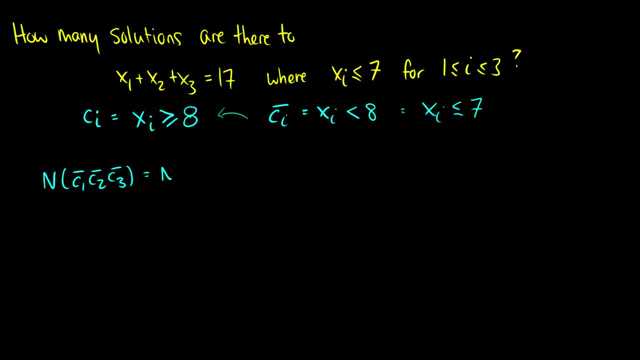 we should know that this is equal to n minus n of c1, plus n of c2, plus n of c3, and then we add back all of the pairs, so plus n c1, c2, plus n c1, c3, plus n c2, c3, and then at the end here we: 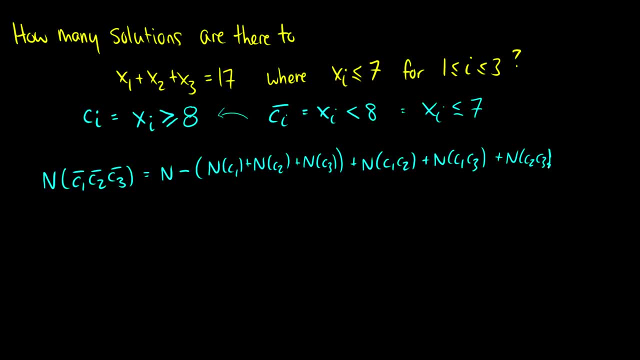 just want to subtract the final condition where it's all of them. so c1, c2, c3.. Okay, well, sometimes it takes a little bit of work to figure things out. I mean, there's a lot of different calculations, so if you're not good at counting, you're going to have problems here. So 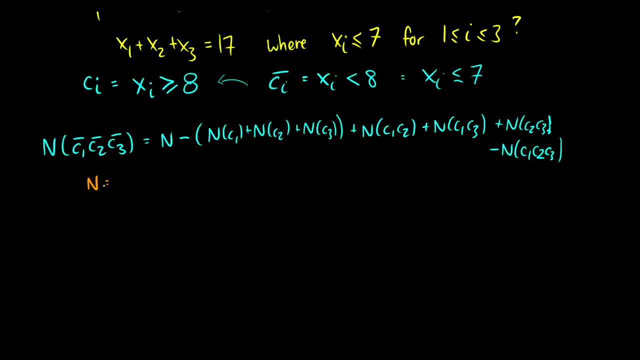 the total amount of solutions we have is just x1 plus x2 plus x3 is equal to 7.. We know from counting that this is equal to 19, choose 17.. This is combinations with repetitions. There are 17 items. we're counting. There are three bins, so we take 3 plus 17 minus 1 choose. 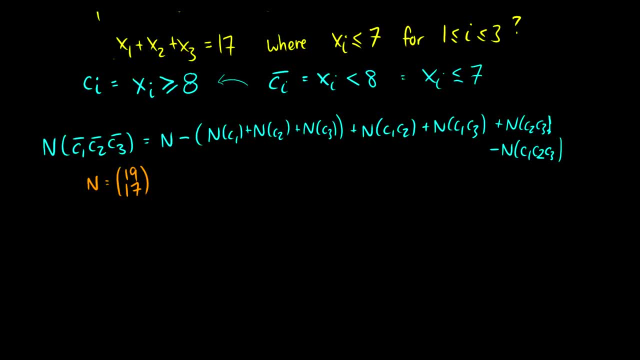 17.. So that's how we get the total amount. Now n of c1. we have the condition where x1 has to be less than or equal to 7, or, sorry, x1 has to be greater than or equal to 8.. So I'm. 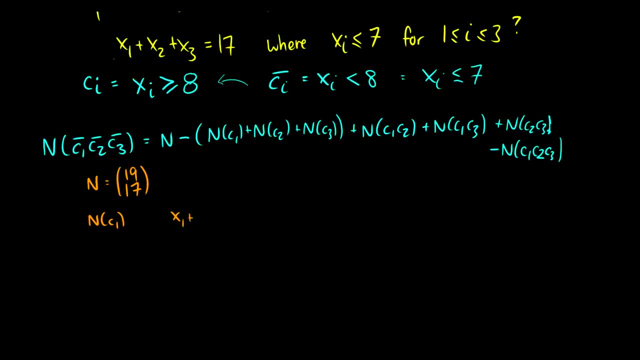 going to write out this first one here. So we have x1 plus x2 plus x3 is equal to 17, and we have x1 has to be greater than 8.. So what we can do is we can substitute this. We can say that x1. 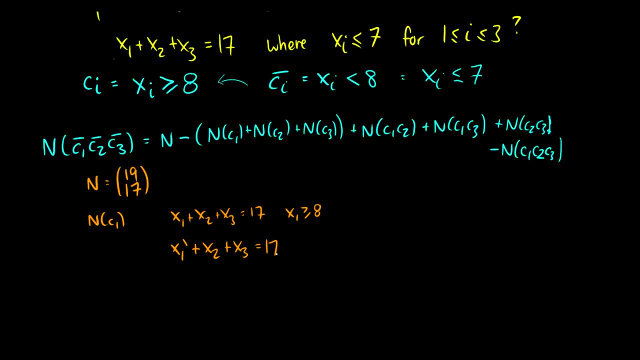 plus x3 is equal to 17 minus 8 and we'll have: x1 prime has to be greater than 0. So this is a way we can substitute it down and still have the same answer, because whatever our x1 prime ends up being, 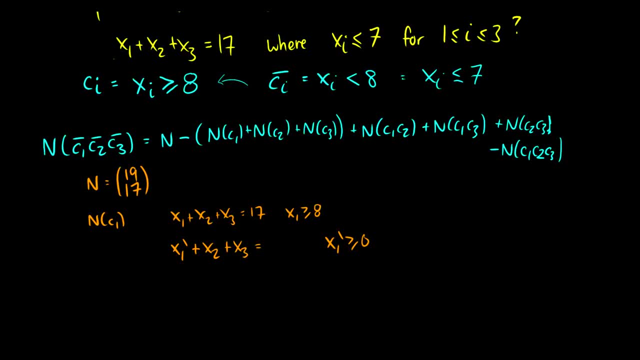 we just add 8 to it. So what we really want is for the rest of them to total 9.. Okay, and this is just the same thing, as 9 plus 3 minus 1 is 11. 9. so, because of our conditions, that all the conditions are the same. So we know. 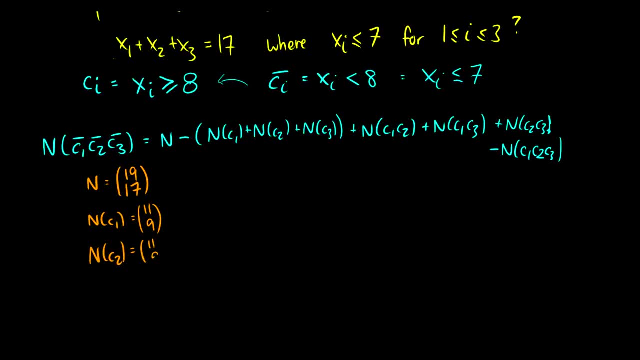 that n of c2 must be the same thing- 11 choose 9- and n of c3 must also be 11 choose 9.. So instead, because all the conditions are the same, we can generalize it a bit. If we can say that n of ci is equal to well, we have. 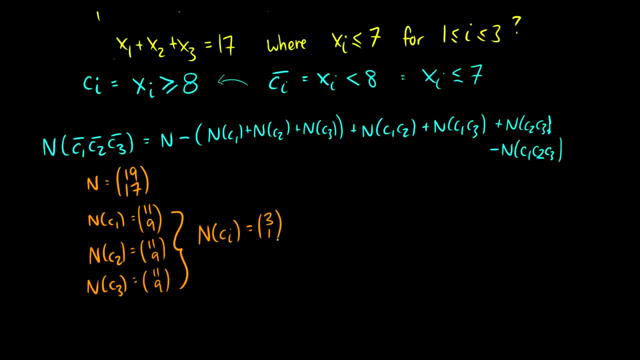 three different conditions. you just pick one of them, and that'll be 11- choose 9.. So you just take three. there are three ways to choose the ith condition, and each condition is 11, choose 9.. Okay, so what about n of c1, c2?? Well, here we have. 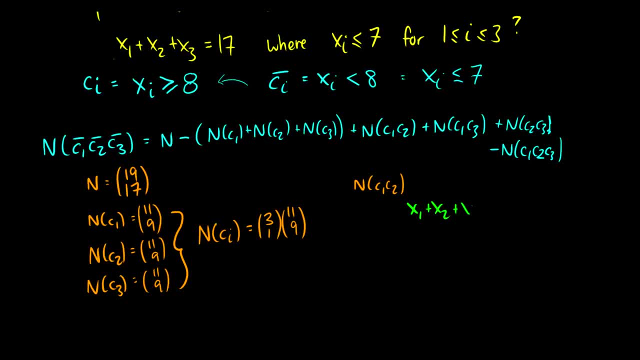 the case where x1 plus x2 plus x3 is equal to 17,. but x1 has to be greater than or equal to 8, and x2 has to be greater than or equal to 8,. so we're going to make some substitutions: x1, prime plus x2, prime plus x3 is equal to. 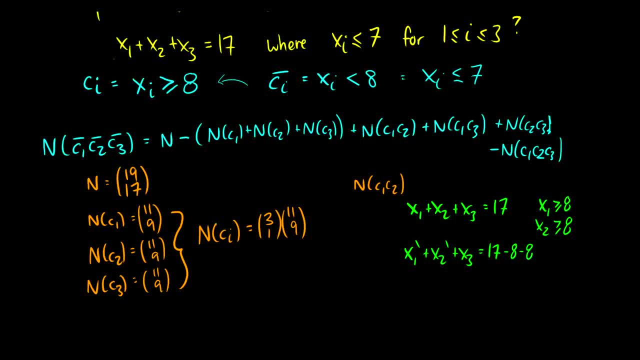 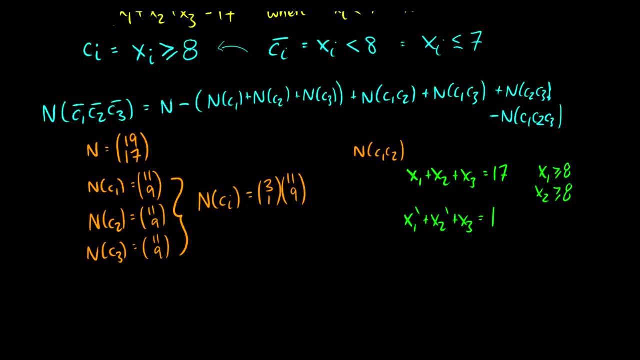 17 minus 8 minus 8, so this is the same thing as 1, same reasoning as before. so now this is going to be equal to 3 plus 1 minus 1 is 3, choose 1, okay, but just like the previous case, because all the conditions are the same, we know that. 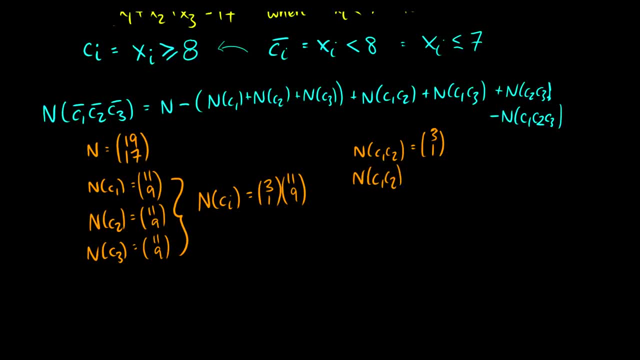 n of c1, c2, or sorry, n of c1, c3 is also going to be 3, choose 1, and n of c2, c3 is also going to be 3,, choose 1.. So once again we can generalize and say that n of ci, cj is just going to be equal. 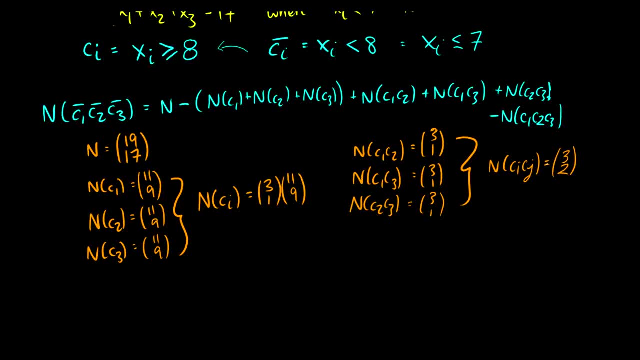 to well, now we choose two conditions out of the three, and each of those is just 3, choose 1.. So we can do that Now for n of c1,, c2, c3, is it possible to have all the x's greater than 8?? 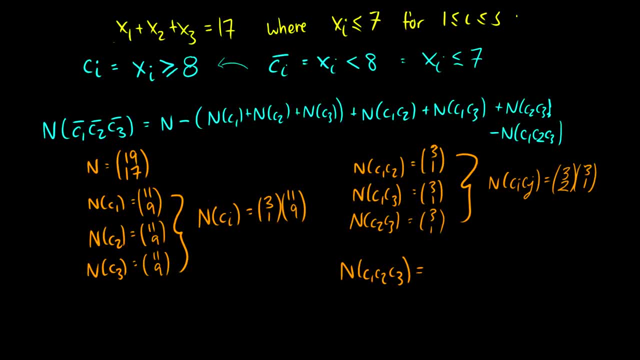 No, it's not possible, because then we'd have x1 plus x2 plus x3. has to be at least 24, and that can't happen, so there's zero ways for all three of these conditions to be met. Okay, so now that we have our numbers here. 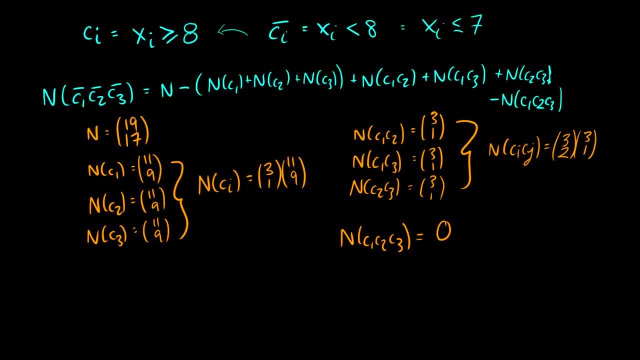 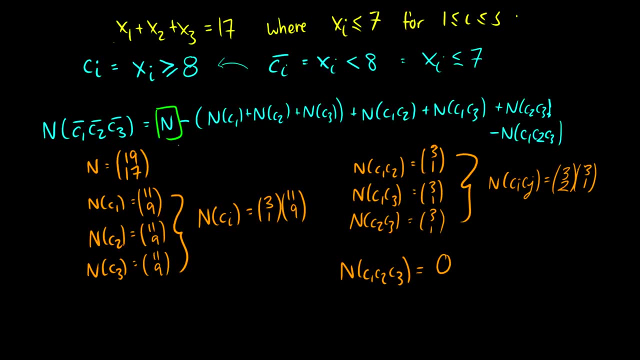 I'm going to introduce some notation I'm going to use. So what we have here is we take n, we're going to relabel this as s0. So this is the number of elements satisfying zero of the conditions. Then we have this big block of n of c1 plus c2 plus c3. 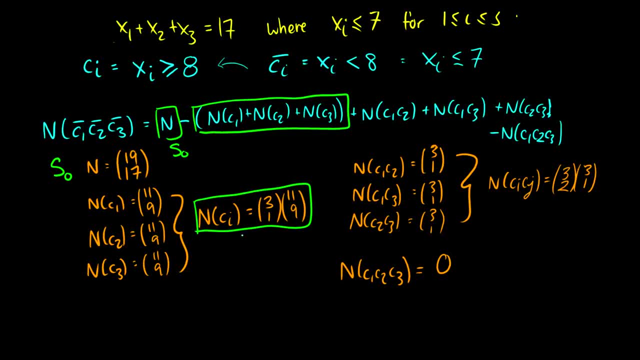 This is the same thing as our n of ci here. We're going to label this as s1 for the number of conditions satisfying x1.. Similarly, for the c1, c2, c1, c3, and c2, c3,, we're going to label this as s2 for the number. 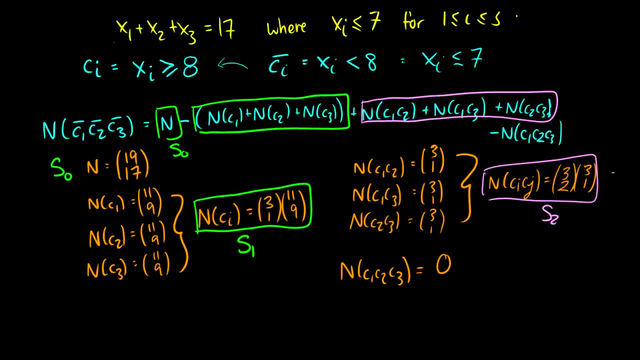 of conditions, or the number of elements satisfying two conditions. And of course, for this last one, you can probably guess we're going to call this k. I'm just kidding. we're going to call this s3,, just to be consistent. So this will be s3, and now we can. 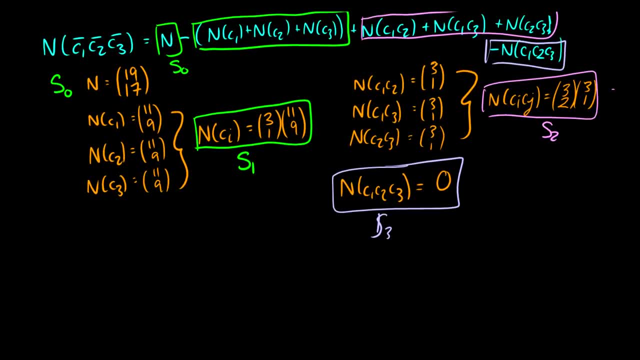 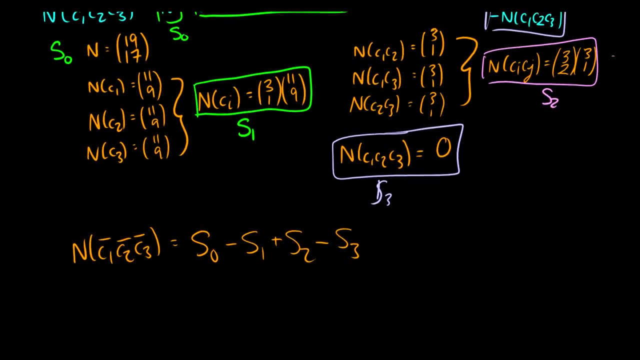 we can write this a little bit nicer. So if we want n of c1 bar, c2 bar, c3 bar, we can just rewrite this as s0 minus s1 plus s2 minus s3.. And now we just plug in the values we got. So our s0 is 19. 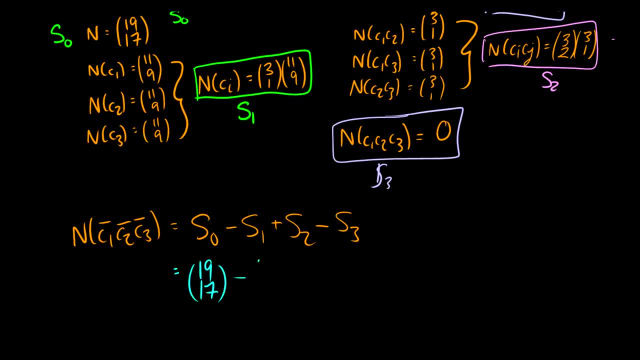 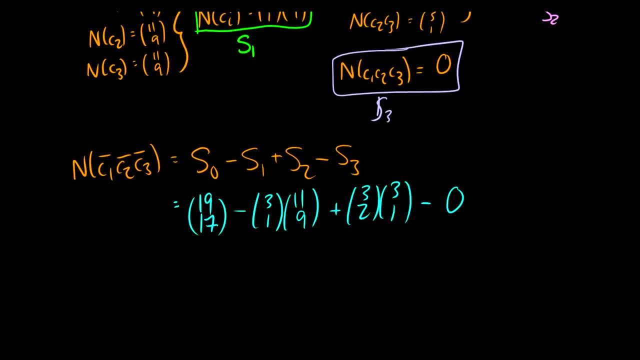 choose 17.. Our s1 is 3- choose 1 times 11- choose 9.. Our s2 is 3- choose 2 times 3- choose 1.. And our s3 is just 0. So this is the number of integer. 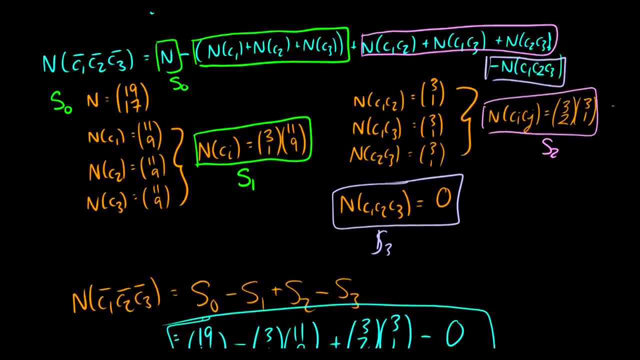 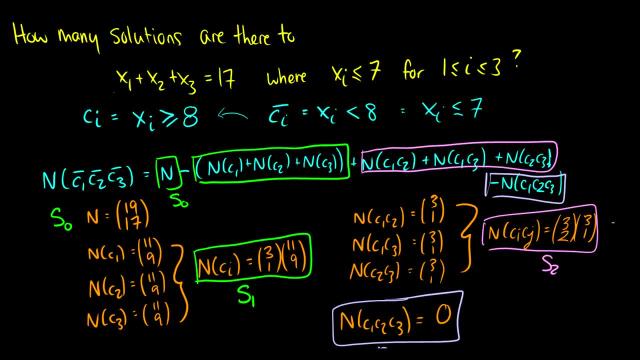 solutions to: x1 plus x2 plus x3 is equal to 17,, where all of our x's have to be less than or equal to 7. So that is a very cool application of the inclusion-exclusion principle. Okay, might not be. 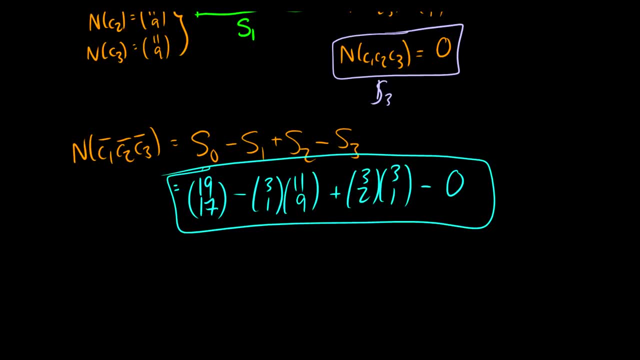 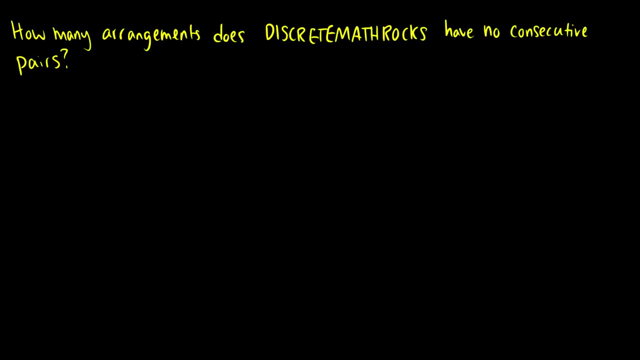 that cool, But trust me, it's. it's pretty cool. So there's one way we can do it. Another thing we can do is we can do letter arrangements. So we have this word: discrete math rocks. it's kind of a weird. 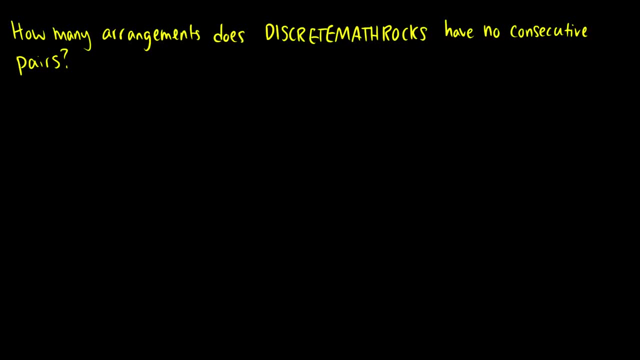 word doesn't make any sense, And we want to know how many arrangements have no consecutive pairs. So what we probably should do is list out all of the letters and make sure that we know how many of them are consecutive. So we're going to do that, And we're going to do that, And we're going to do. 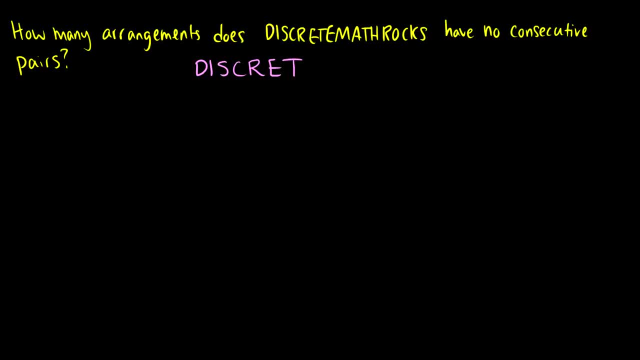 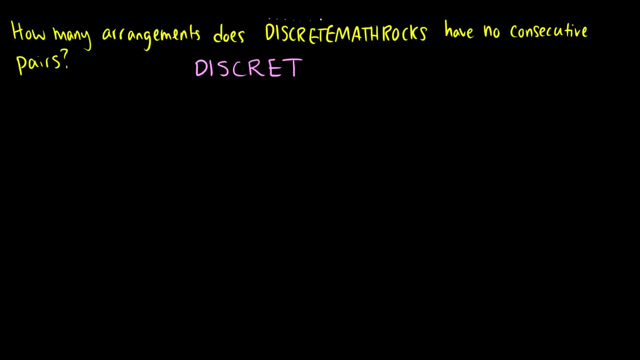 what do we call it? we are thing including something coming. what about an S? Okay, so why do we do this? We need to know which or how many of each letter there are, so that way we don't count them as two different scenarios. Because, if you remember, 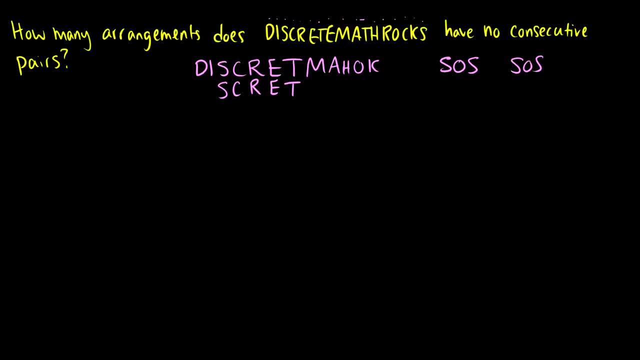 we have the word SOS and SOS. These might be different S's, but they still count as the same word, so we don't want to count those twice. Okay, this is why I did counting review, because you need to know these very well. So how many arrangements does this word have? no consecutive. 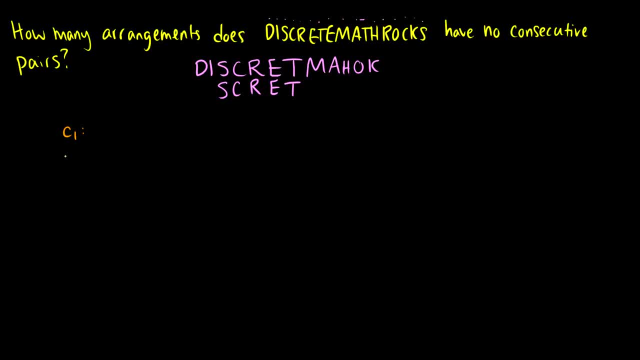 pairs. Well, what are our conditions? Condition 1 is going to be that SS is together, because that's a pair. C2 is going to be CC. it's going to be together. Condition 3 will be the R, the R, C4. 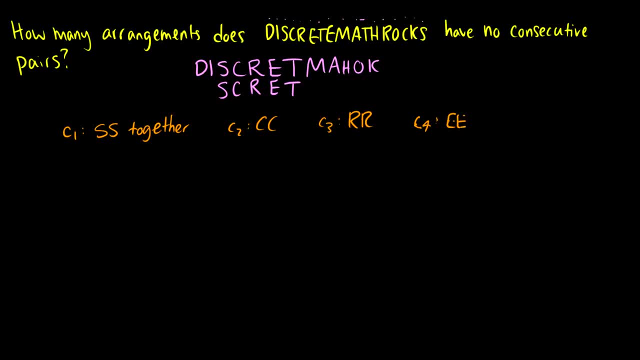 is going to be. So now we want N of C1 bar, C2 bar, C3 bar, C4 bar and C5 bar. This could be a really long question, but we know this is just going to be S0 minus S1 plus S2 minus S3.. 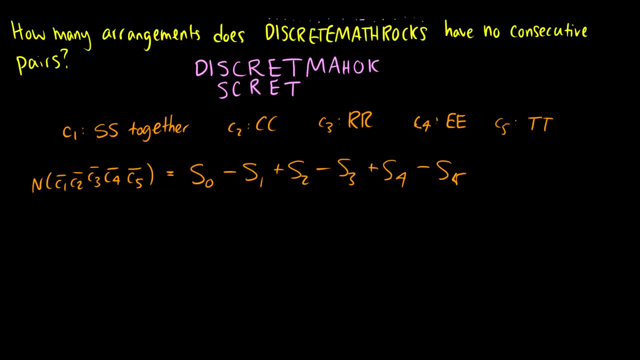 Plus S4, minus S5.. So this is why I introduced the notation, because we're going to need this. The nice thing about this is that all of the conditions satisfy the same equation. So if we pick any one condition, it doesn't matter which one we pick. they're all going to give us the. 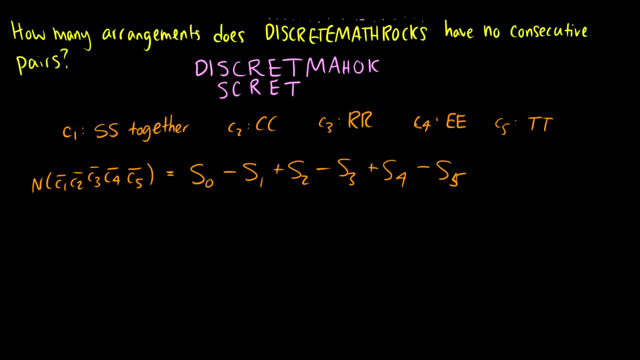 same results, And that is why this formula works much nicer. So how many total ways are there to arrange all the letters here without any restrictions? Well, how many letters are there? 1, 2,, 3,, 4,, 5, 6,, 7,, 8,, 9,, 10,, 11,, 12,, 13,, 14,, 15, 16.. There's 17 total letters, So we can arrange. 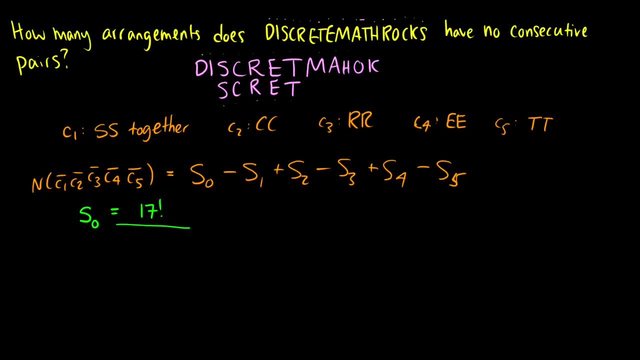 those 17 factorial times. Okay, now there's two S's, so we have to divide by two factorial. Two C's, so we divide by two factorial. And of course we have five pairs, so we have to divide by two factorial five times. Okay, now S1,. well, to pick one condition, there's five. 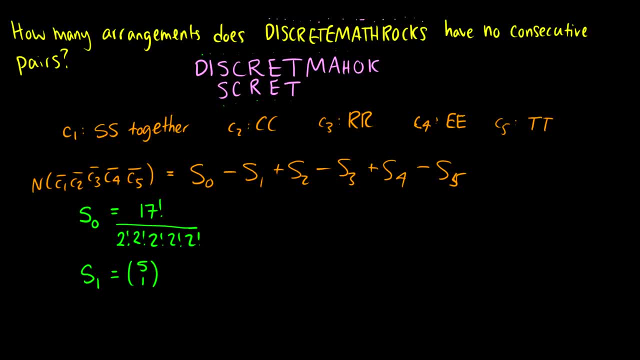 choose one ways. we can pick one of the five conditions. And let's say, for instance, that the SS is together. So instead of listing them as two separate letters, we're going to list them as a pair together. So we're going to treat SS as a pair. So we're going to treat SS as a pair. 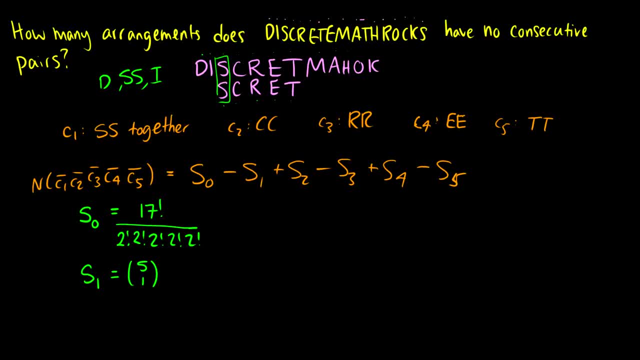 So we're going to treat SS as if it's one letter. So this leaves our total here at 16 factorial letters to choose from, And there's no longer five pairs that are repeating. There's only four pairs that are repeating because we're treating this as one item, while these two C's here would 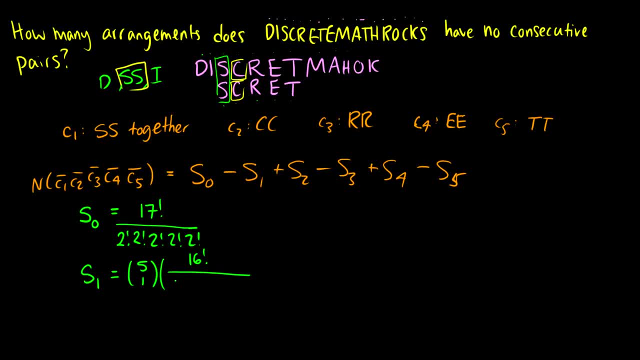 still be separate items. So we have 16 factorial divided by two factorial four times four times. Okay, so that's S1.. Now if we did the same thing with the C's as one unit, we'd have the same. 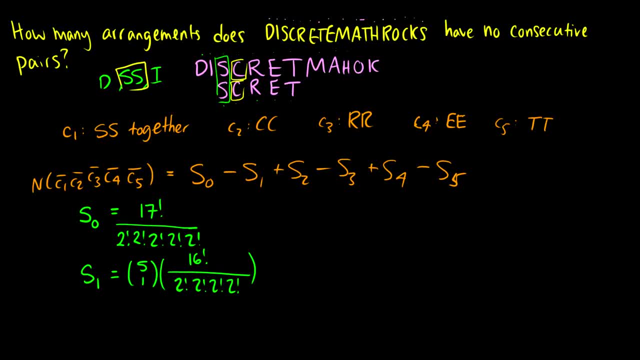 result. So we can do this with all five conditions, And that's where this five choose one is coming from. Okay, what about S2?? Well, S2, now we just pick two out of the five conditions. So that's five. 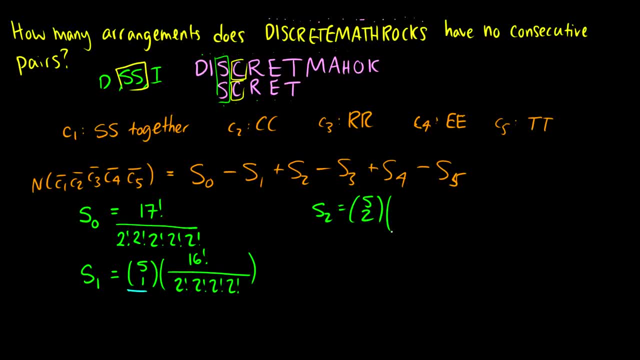 choose two And we repeat the same process. So now we take, say, RR and EE to be one item, So then we get 15 total letters to choose from And we divide by two factorial three times. Okay, what about S3?? Well, S3 is just going to be five. choose three. 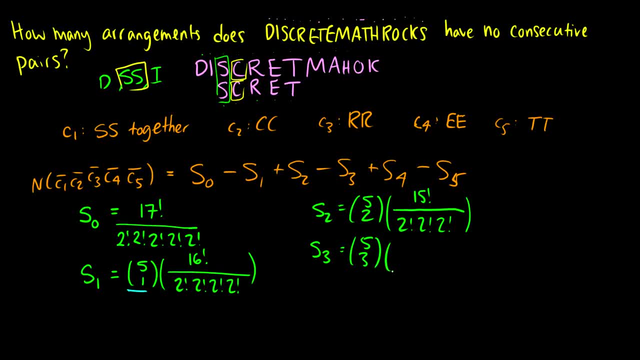 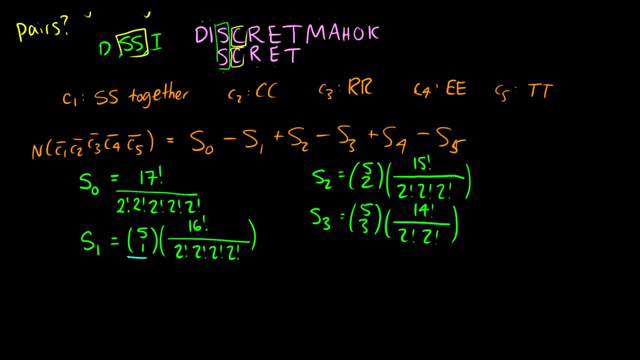 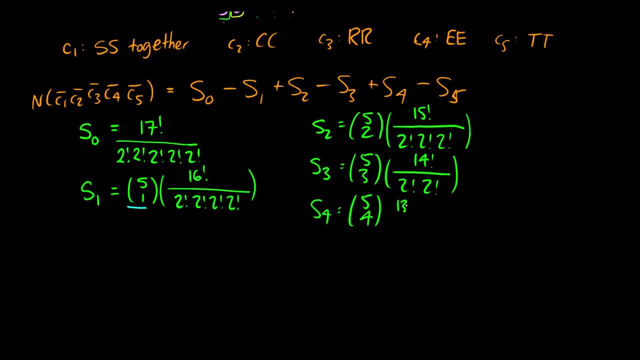 because now we're choosing three out of the five conditions And this will be 14: factorial over two factorial, two factorial- Hopefully you see the pattern now. Then S4 is going to be five. choose four Times 13: factorial over two factorial And then S5 will finally be five. choose five And then 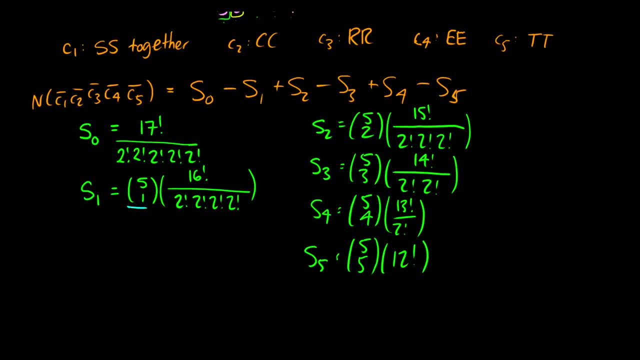 there's just 12 sets of letters remain. So this is your answer. I'm not going to write it all out in one lump, because here is the answer And we have all the individual parts here, So there's really no need for me to write it all out. In fact, if you don't want to, on a test it's probably. 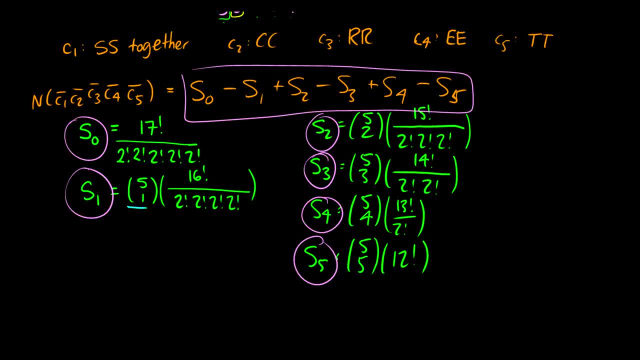 okay, Because it's just simple substitution. at this point There's no point in simplifying it. If you're in a course with a calculator, I'm so sorry because it's just a lot of wasted time. So that is letter arrangements. Pretty cool. Here's another question. Here's a word problem. 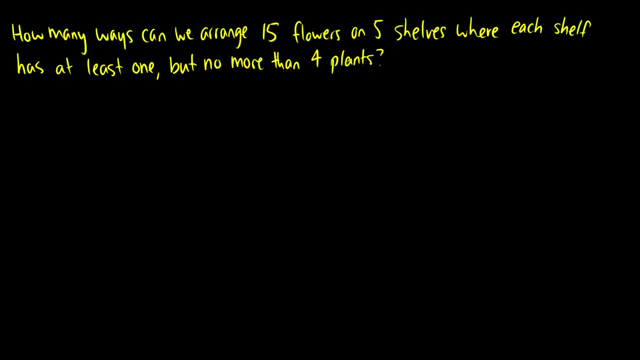 And this might seem tricky at first, but I'm going to show you that it's actually pretty obvious. In fact, we've already done this in this video: How many ways can we arrange 15 flowers on five shelves, where each shelf has at least one, but no more than four plants? So if we have five shelves, here we have. 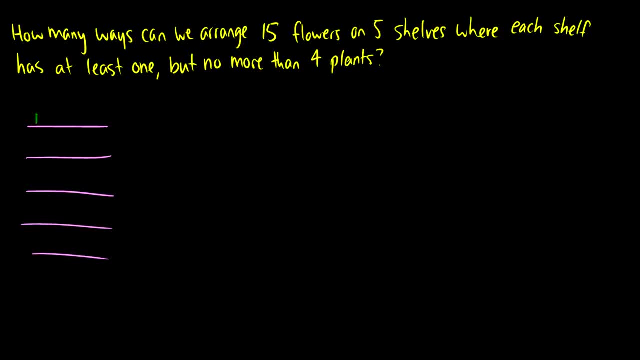 15 plants, So we can put. you know, we have to have at least one on each shelf, So that's good, And then we probably have to distribute. So we have five here, So we have 10 left, So we have to put a bunch on shelves, but we can't ever have more than four, So we can do. 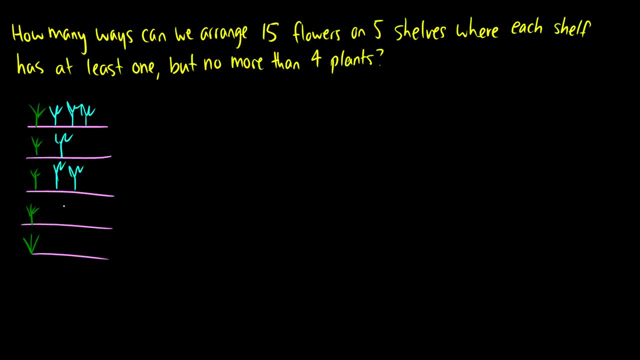 this. So we have 1, 2,, 3,, 4, 5, 6.. Put three on this one And we can put one on this one. So that's one arrangement we can do. Now. this is the same thing as solving x1 plus x2 plus x3 plus x4. 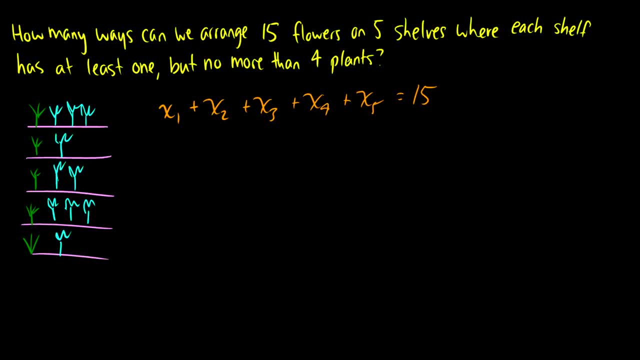 plus x5 is equal to 15.. We just have the first shelf here, the second shelf, the third shelf, the fourth shelf and the fifth shelf, And we have some restrictions where xi has to be between 1 and 4. So we can augment. 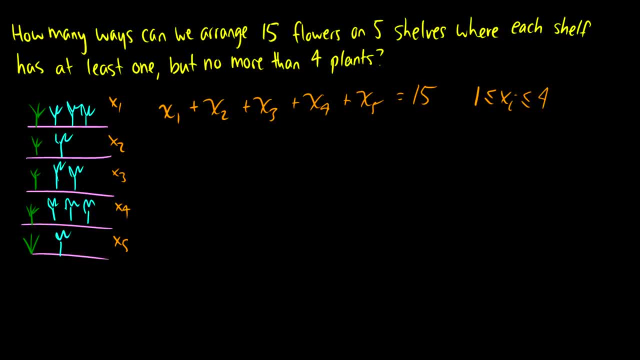 this a little bit to make it a little bit easier for us, because we don't like this greater than or equal to 1 here. So we'll make some substitutions. We'll say: okay, now we have x1 prime, x2 prime, dot, dot, dot all the way up to x5 prime, And this is going to equal 10,. 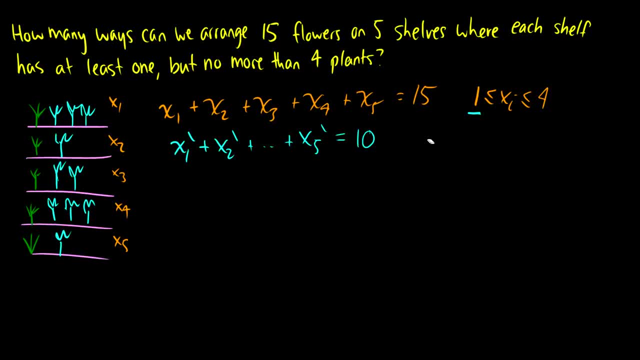 where now xi just has to be less than or equal to 3.. Because we just basically shift one down from each. And this makes sense, because when we put one on each shelf we only had 10 remaining plants to choose from. So this equation follows very nicely from a die. 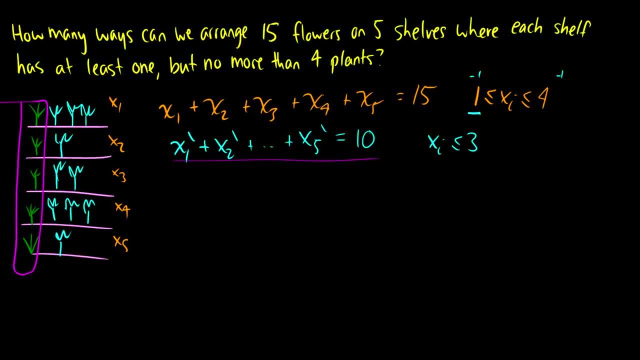 Okay, well, you remember what we did before. right, Try to solve the rest of this on your own, But if not, you can follow along here. Well, ci is going to be. xi is greater than or equal to 4.. 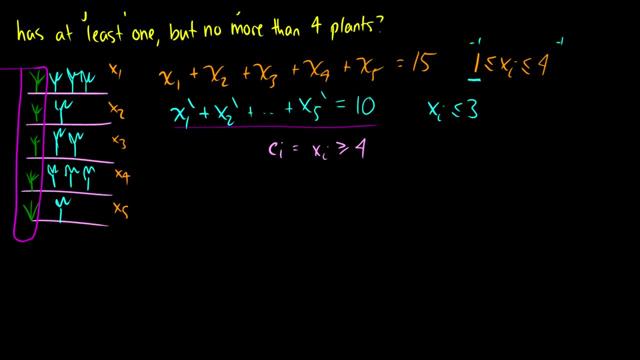 That's going to be our conditions. So that means that, well, if we want not c1,, c2, c3.. I really don't know why this does this on the laptop sometimes. Okay, then we want C4 bar, C5 bar. Well, again. 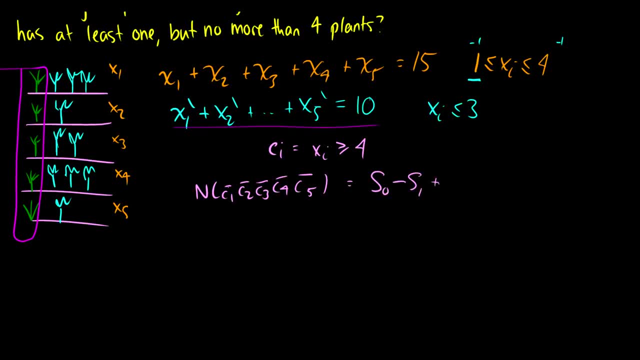 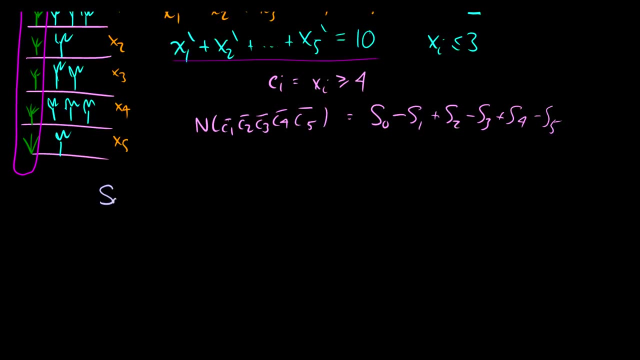 we know this is the same thing as S0 minus S1 plus S2 minus S3, plus S4 minus S5, so it takes a lot of time. Okay, let's do this step by step. So S0 is just the total number of. 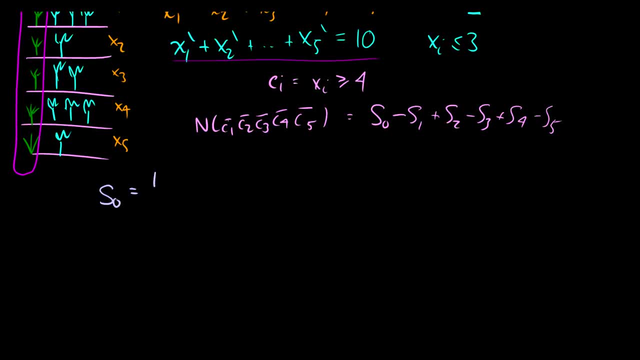 solutions there are to this equation, So this will be 14. choose 10. for the same reason as before: Pick 10 items. There are 5 bins, so we need 4 dividers. so that's 10 plus 4 is 14.. Choose 10.. 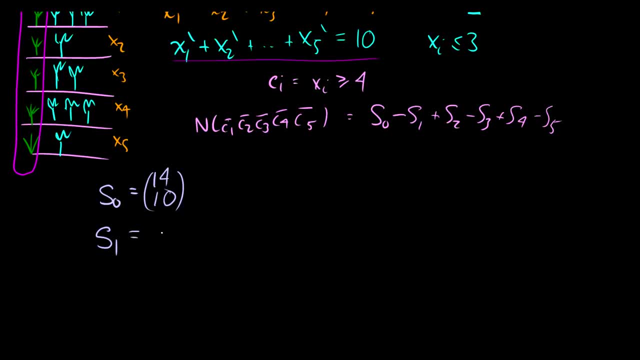 Okay, S1.. Well, we have to choose one out of the five conditions. so 5 choose 1.. And now we have: xi is greater than or equal to 4.. So we're going to have to make another substitution here, If you. 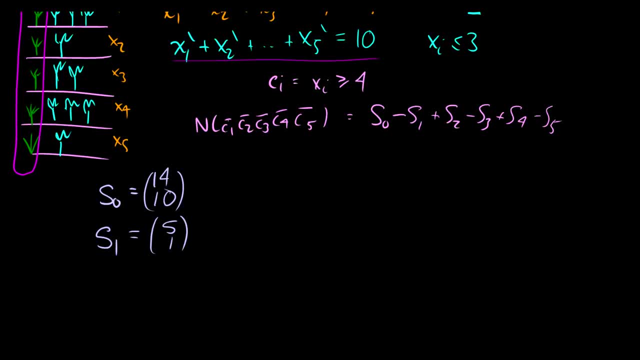 follow the same reasoning as before. I'm only going to write this one out: once We'll have x1, we'll call this prime. prime plus x2, prime plus x3, prime plus all the way up to x5. prime is going to equal 10 minus 4, because we made this substitution here with x1. 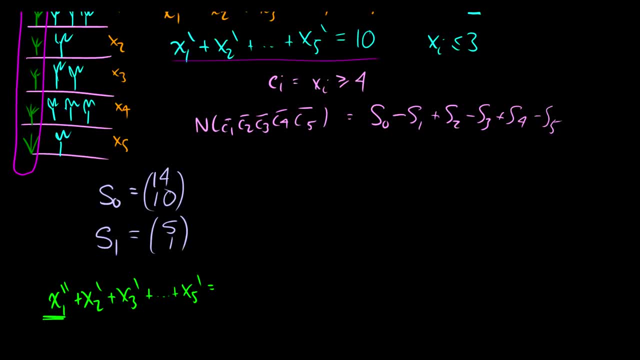 greater than or equal to 4, so this will be equal to 6.. Therefore, s1 will be 11 minus 1 is 10, choose 6.. Okay, now s2, we can just apply the same reasoning here. This will be 5, choose 2. 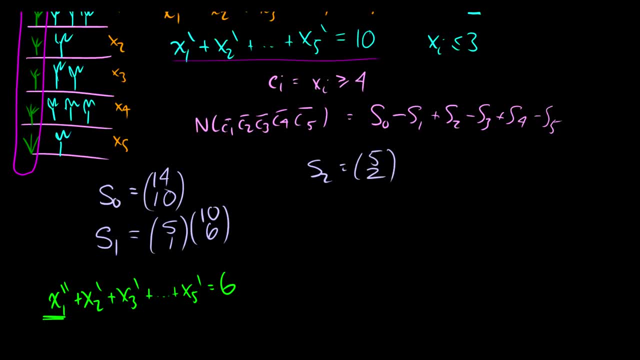 elements, and if you see a pattern here that makes a jump here, it's probably going to make the same jump and you can verify for yourself that it does so. but if we have so, 14 to 10, we subtract 4 on the top, 10 goes to 6, we subtract 4 on the bottom, so this will be. 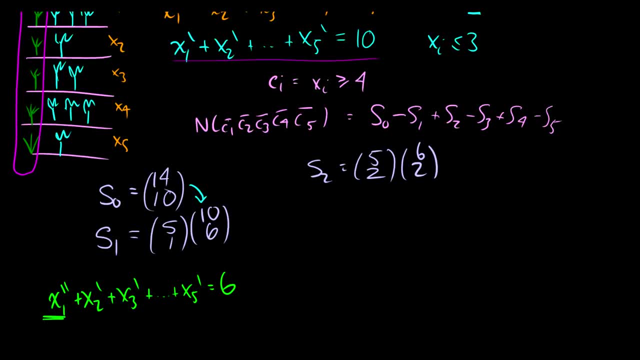 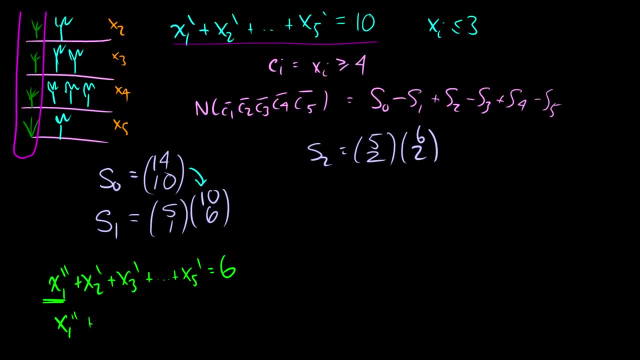 5, choose 2 times 6, choose 2.. In fact, for the sake of completion, let's see what x1 prime prime is going to do. So if we have x1 prime prime, we subtract 4 on the top, and if we have 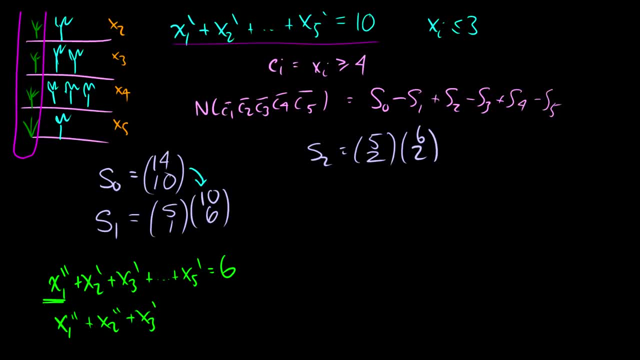 x2 prime prime plus x2 prime prime plus x3 prime plus x4 prime plus x5 prime is going to equal 6 minus 4, which is 2, so this will be 5 plus 2 minus 1 is 6, choose 2, so s2 is going to be 5, choose 2. 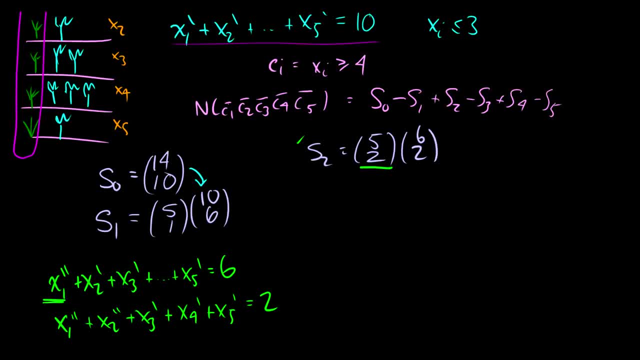 times 6 choose 2.. Again, 5 choose 2, because we're choosing 2 out of the 5. conditions: Okay, s3.. Well, if you've been paying attention, you should know that s3 is not possible. You. 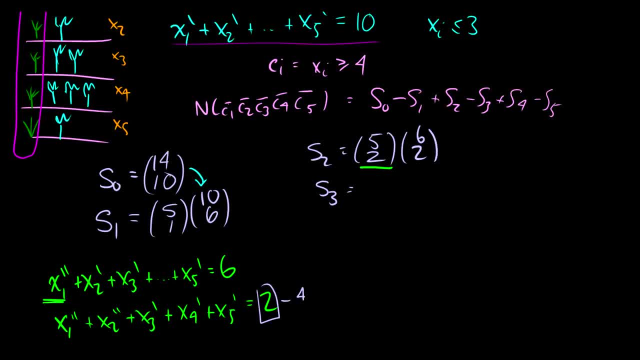 should know that s3 is not possible because if we subtract another 4, then this has to equal negative 2, and that can't happen. We can't have positive integers equaling negative 2, so s3 is going to be 0, which means that s4 should be 0, and s5 should be 0. There's no way. 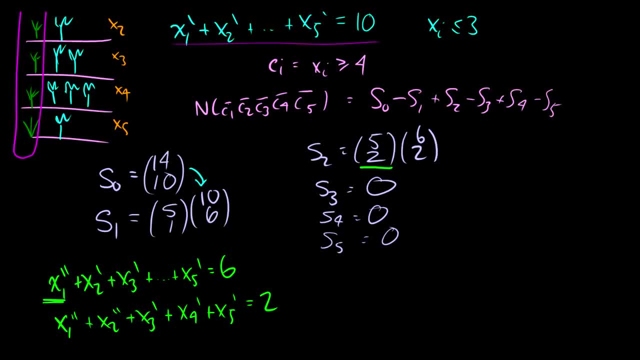 to have three or more of these conditions satisfied. So our result is going to be 14- choose 2 times 6.. 5- choose 10 minus 5. choose 1 times 10. choose 6 plus 5. choose 2 times 6, choose 2.. So this is the. 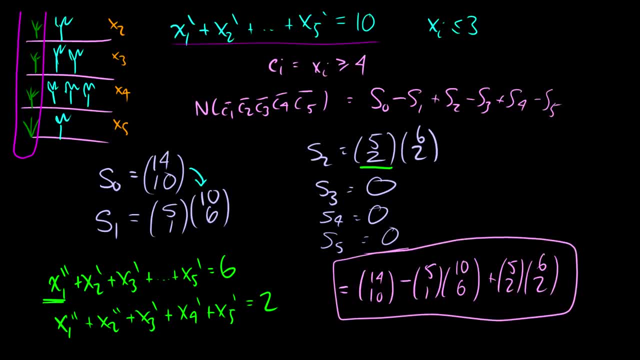 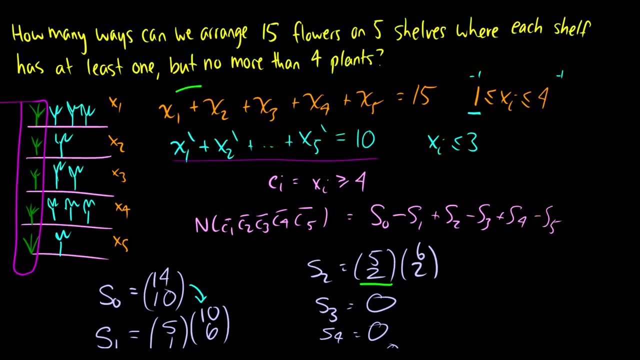 number of ways you can arrange 15 flowers on 5 shelves, where each shelf can have between 1 and 4 plants. So that is that question. So if you have a word problem, a good trick is to change it to an equation with conditions. 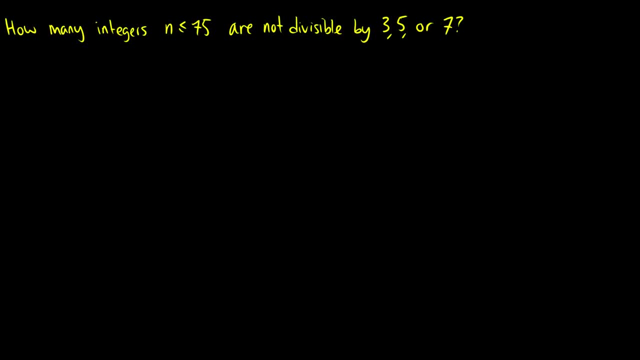 and you can solve it as such. Now here's a question. we've already done sort of. I've changed the numbers a little bit, so do try this yourself. Hopefully it's not too bad. But how many integers less than 75 are not divisible by 3,, 5, or 7? So we want condition. 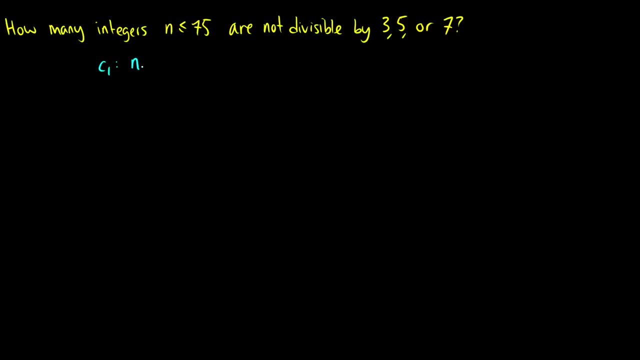 1. We want a number n. I guess we'll do that. Let's do this this way: C1 will have 3 divides n, C2 is going to be 5 divides n And C3 is going to be 7 divides n. 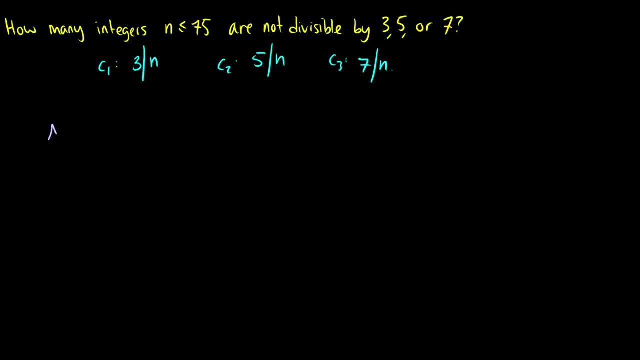 Okay. well, we want n of C1,, C2, C3, each with bars. So how many elements do we have total? Well, 75 total. Then we're going to subtract. well, how many elements divide or are divisible by? 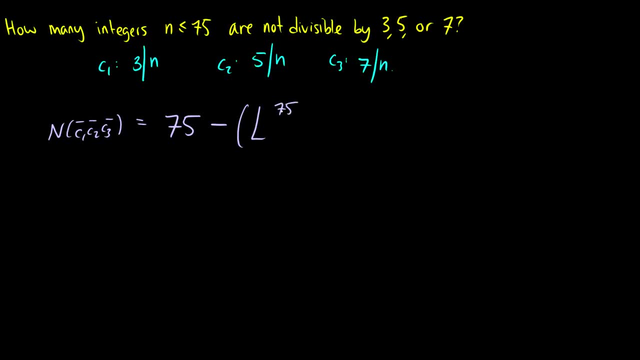 3?? Well, that's going to be the floor of 75 divided by 3.. Then, how many elements are divisible by 5?? Well, that's going to be the floor of 75 over 5.. Divisible by 7 is going to be 75 over 7.. 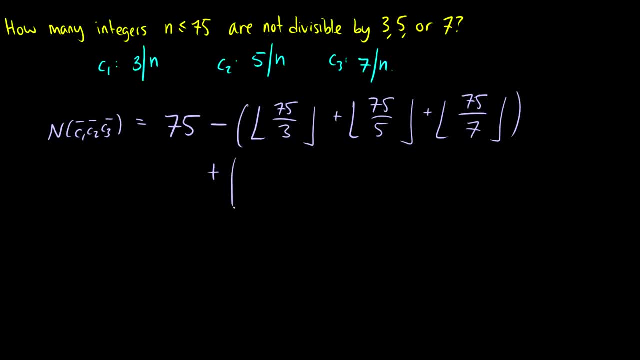 Okay, Then we add back all the pairs, So divisible by 3 and 5 is going to be 75 over 3 times 5.. Take the floor of that. Then we have divisible by 3 and 7.. 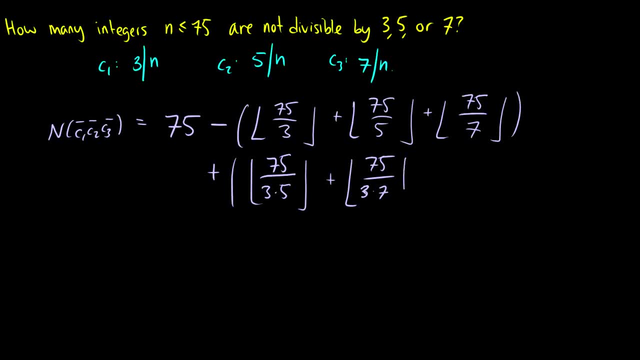 So that'll be 3 times 7.. Then we want divisible by 5 or 7. So that's 75 divided by 5 times 7.. Then of course we add back all the numbers that are divisible by all 3.. 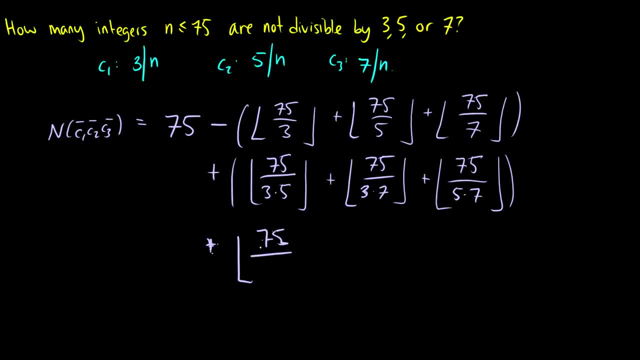 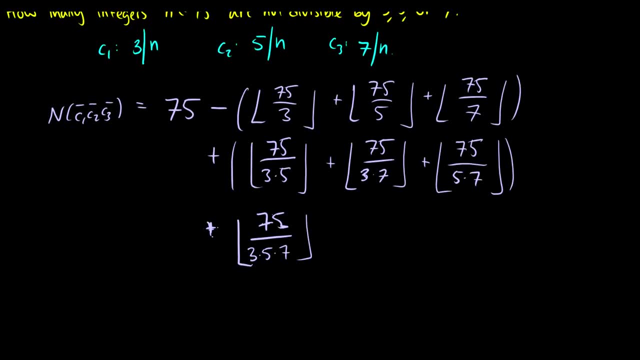 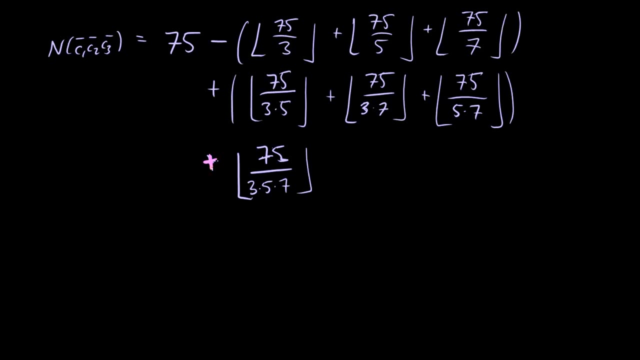 So that'll be the floor of 75 over 3 times 5 times 7.. So this is our answer, but again, we can simplify it a little bit. If you want a full explanation for this question, check out the previous video. 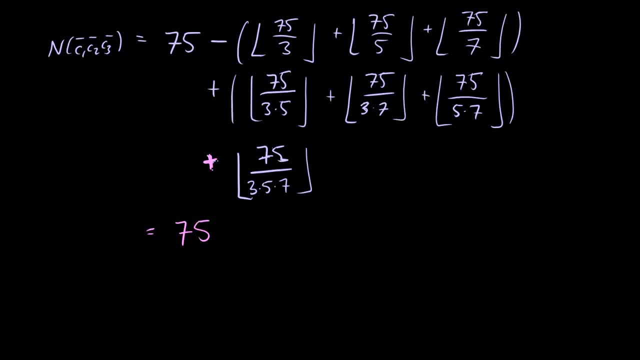 So we have 75 minus. So 75 divided by 3 is going to be 25.. Then we're going to subtract 75 divided by 5, which is 15.. 75 divided by 7 is going to be 10.7271,. 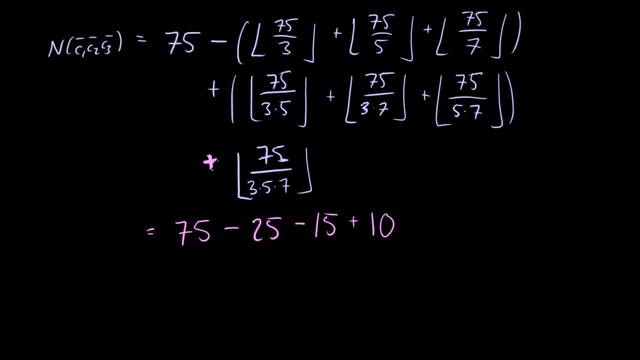 but it's still going to be about 10 because we take the floor. I hope that should be a subtraction. Then we're going to add back 75 divided by 15, which is 5.. Add back 75 divided by 21,, which is going to be 3 and a bit. 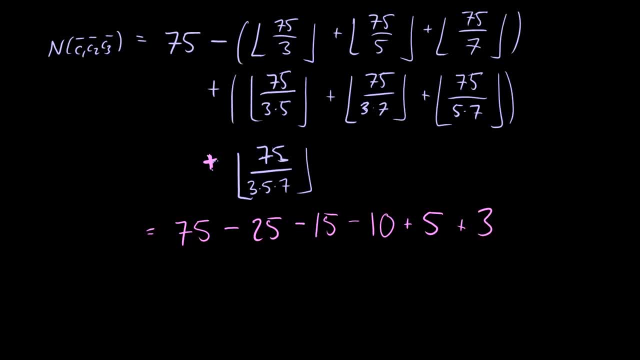 So we add back 3.. 75 divided by 35 is 2.. And then we should be subtracting this last one. We'll subtract 75 divided by 105, which is just clearly 0.. Okay, So this is going to be 75 minus 50 plus 10, which is just equal to 35. 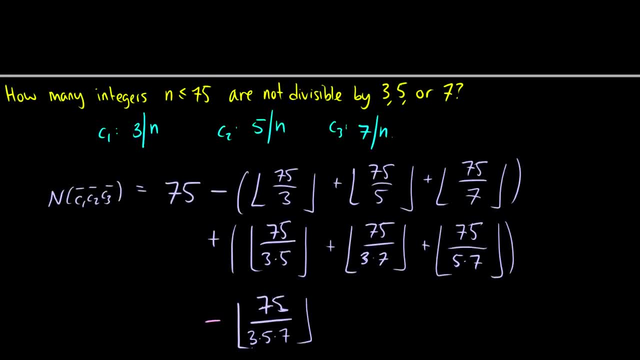 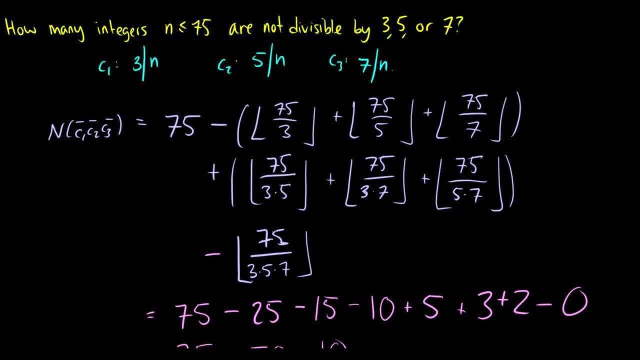 So there are 35 numbers less than 75 that are not divisible by 3,, 5, or 7.. That's kind of cool, because that's more numbers than the amount of numbers less than 100 not divisible by 2,, 3, or 5.. 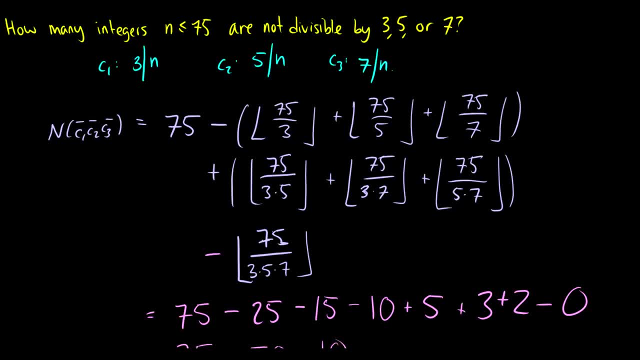 Kind of interesting. So that was some inclusion-exclusion practice. If you have any questions, please leave them in the comments below. I will be happy to type a response or, if the demand is great enough, make a new video If you have any more practice questions related to this that you're not quite sure how to do. 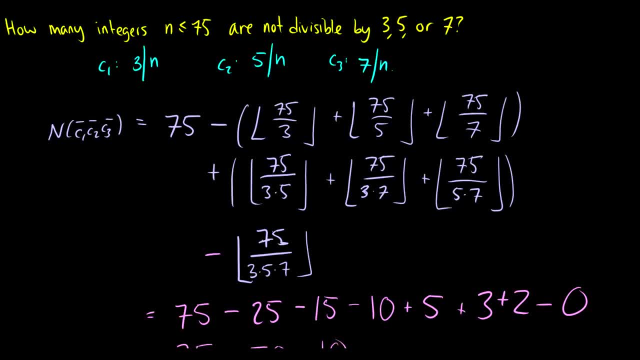 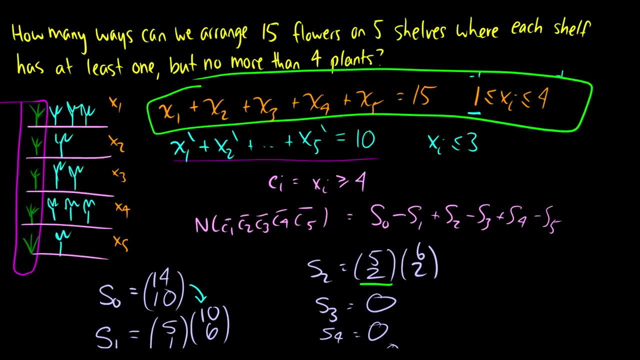 it's also a great place to post them. I think I've covered the basis of most questions that would be answered, But if not, then leave them below and I will see what I can do If I write a practice exam for this course. honestly, this question right here, this flower arrangement question. 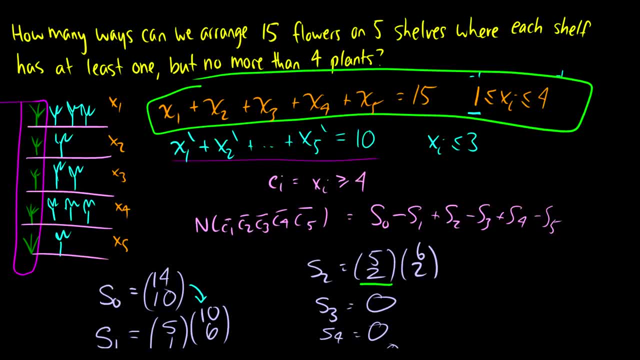 expect something very similar to it, In fact, for an exam. this is a very good question for inclusion-exclusion on an exam, because it requires you to abstract it to this level here, to this equation, and then solve it. You'll normally see this question or you'll see the division question.